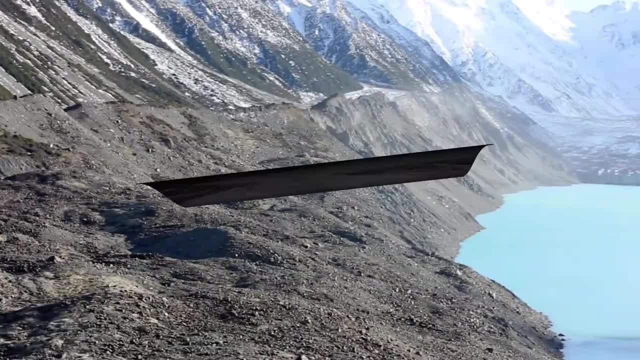 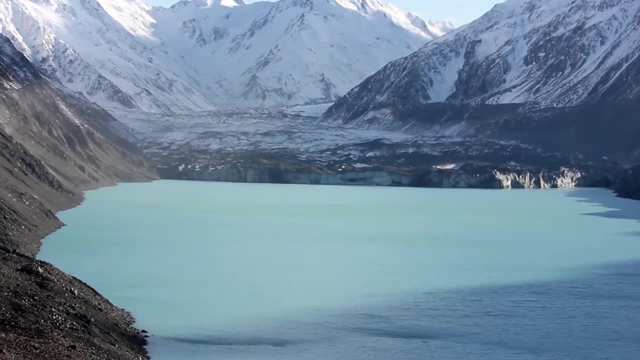 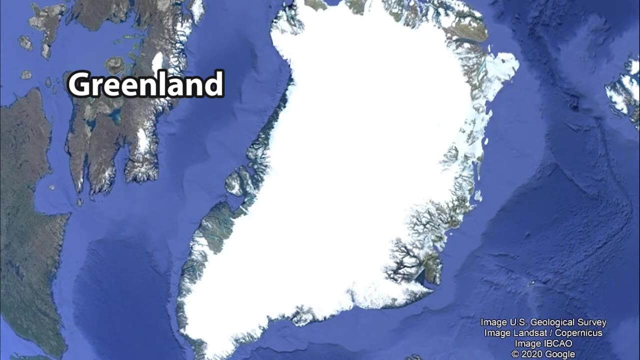 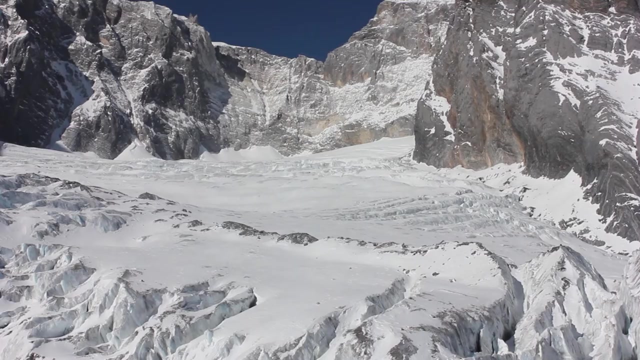 A glacier is a moving river of ice on land. There are two types of glacier. Continental glaciers are massive amounts of ice that cover continents such as Antarctica or Greenland. 95% of ice on earth is locked up in continental glaciers. Alpine glaciers are formed in mountainous 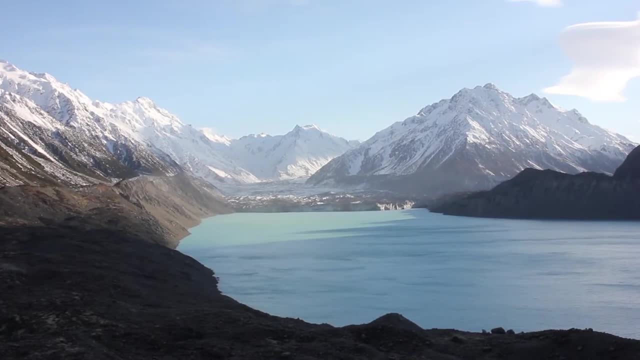 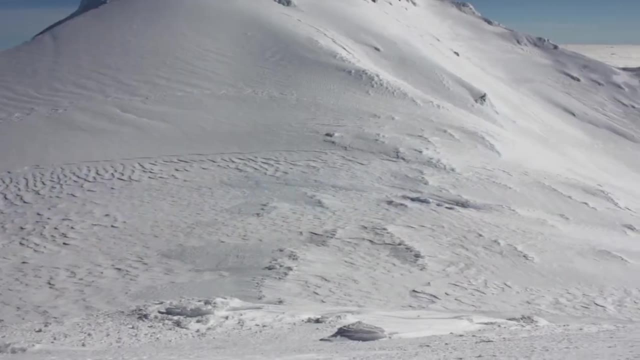 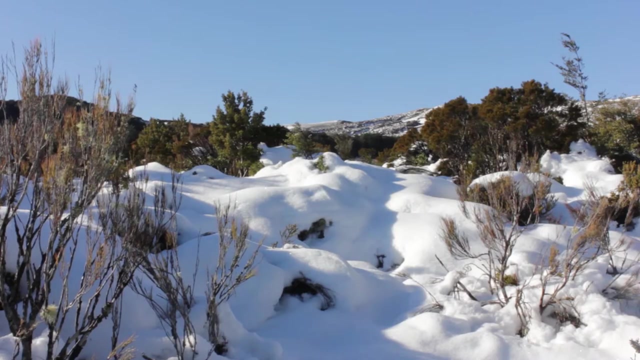 regions. Most of New Zealand's largest glaciers are in the Southern Alps, which have the highest mountains and the heaviest precipitation. Glaciers originate from heavy snowfalls over a long period of time. When snow initially falls, it has many air spaces between the snowflakes. 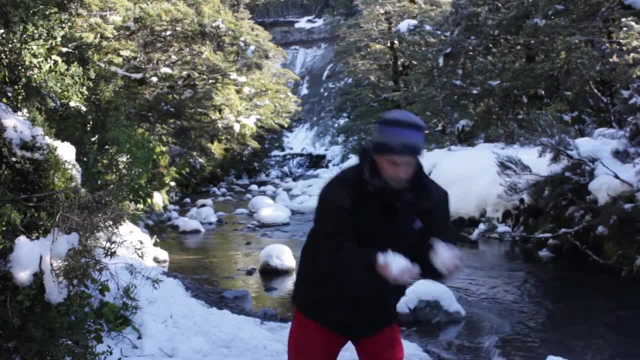 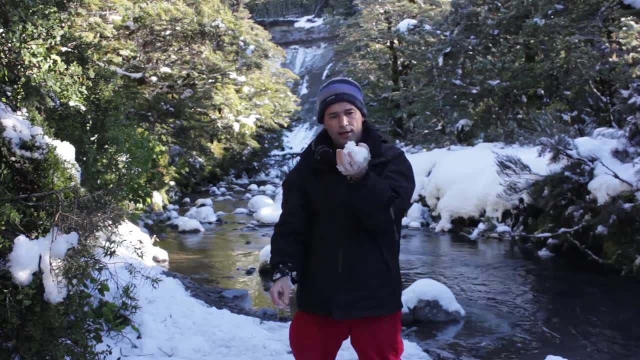 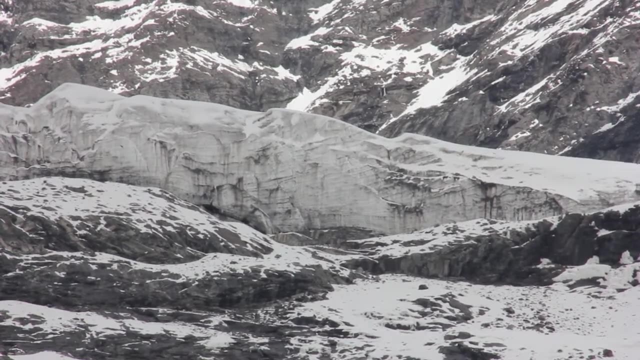 Over time, the weight of new snow above it squeezes the air out of the pore spaces and compacts the snow, just like me, making this snowball. Eventually, this compaction causes the snow to become ice, Because the air is being squeezed out. the ice will turn a bluish. 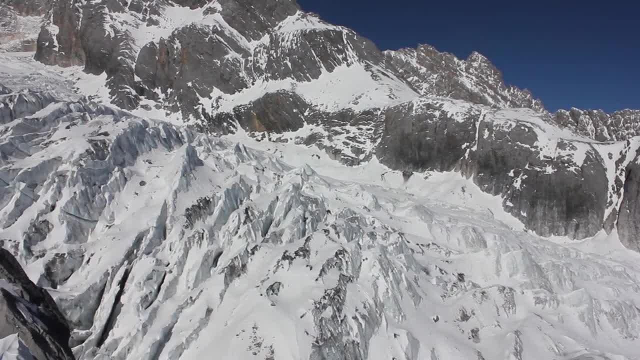 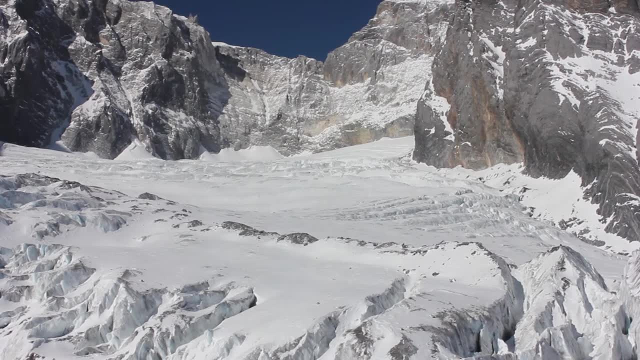 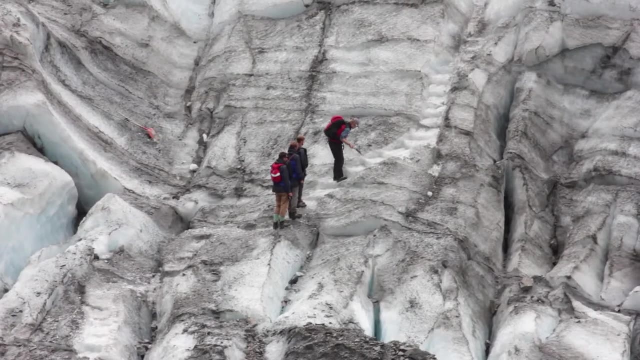 colour Glaciers have several components. The area where the snow falls is usually the part of the glacier with the highest elevation and is called the zone of accumulation. Further down the glacier is the zone of ablation, where most of the melting and evaporation. 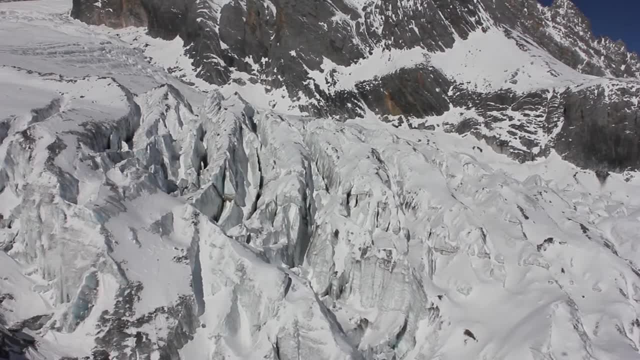 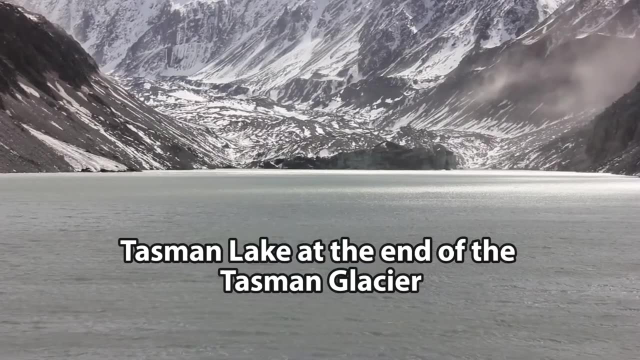 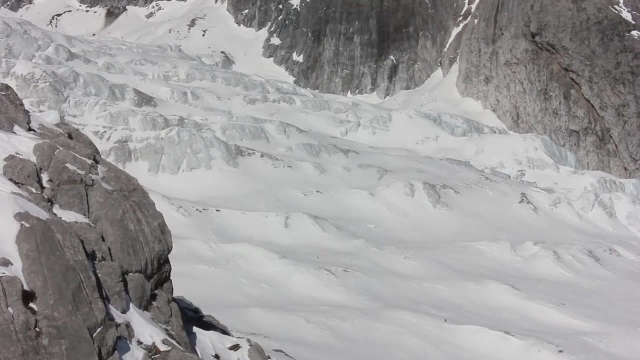 occurs Here. the ice shows a lot of crevasses. The end of the glacier is called the terminus, or snout. At many glaciers there are glacial lakes and the terminus. A glacier will continue to grow as long as the rate of ice formation in the zone of accumulation is greater than. 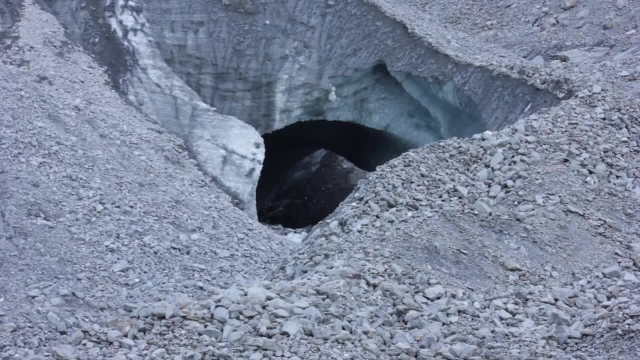 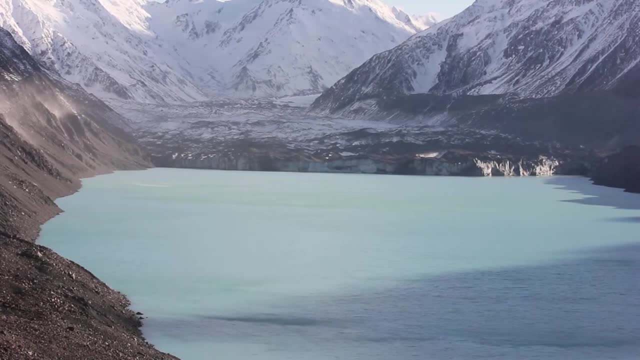 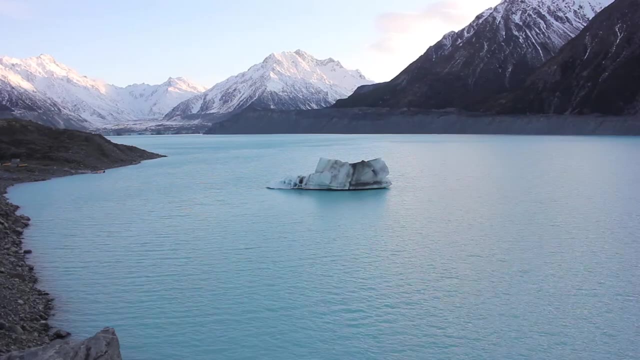 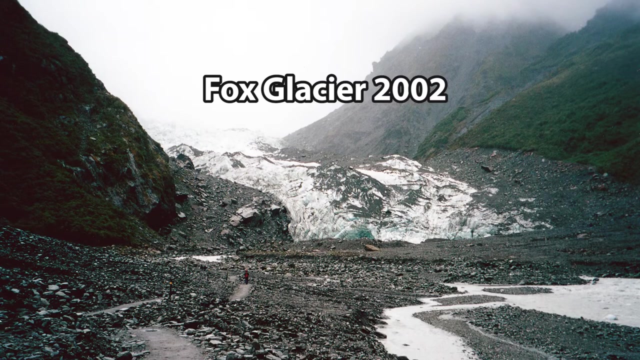 the rate of ice melting in the zone of ablation. When more melting takes place than ice forming, the glacier is said to be in retreat. The Tasman glacier, for example, has been in retreat, causing the Tasman lake to grow increasingly larger. In 1973, this lake did not exist. 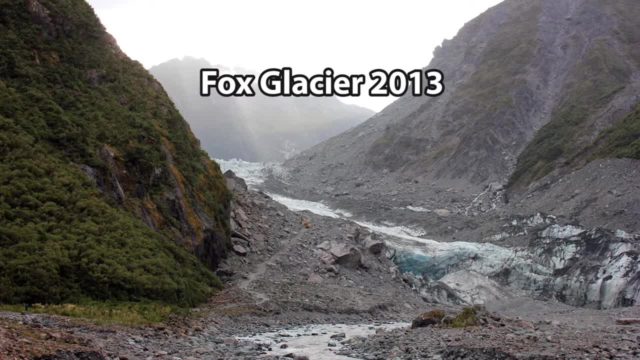 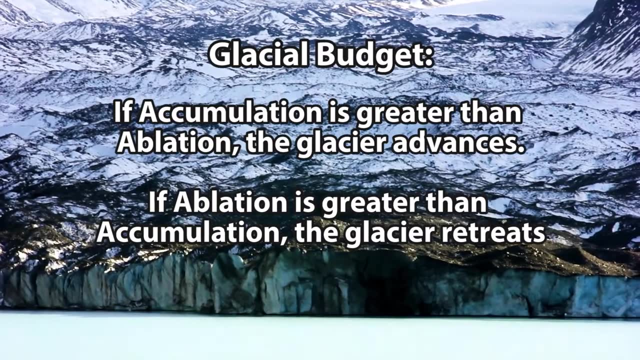 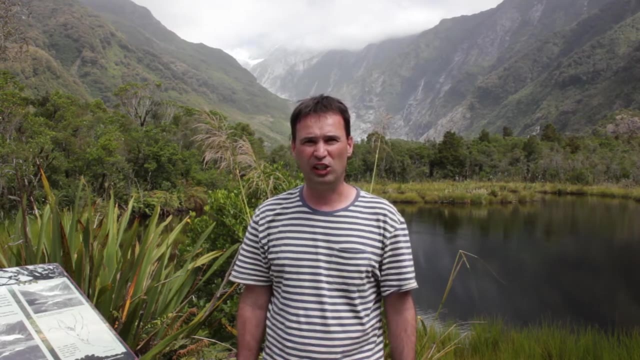 Over a single year, a glacier may both grow and retreat, depending on the rate of accumulation. Over a single year, a glacier may both grow and retreat depending on the rate of accumulation. This is called the glacial budget. In times when global climate has been cooler, glaciers have expanded. We call these periods. 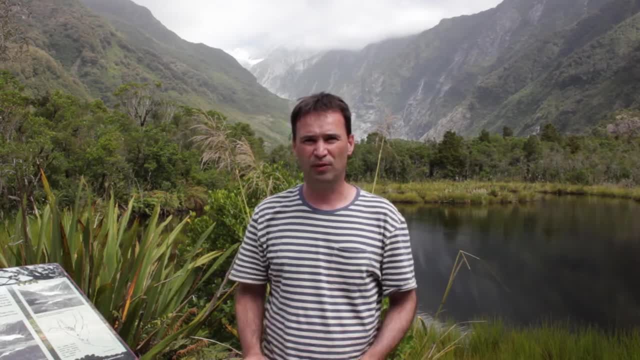 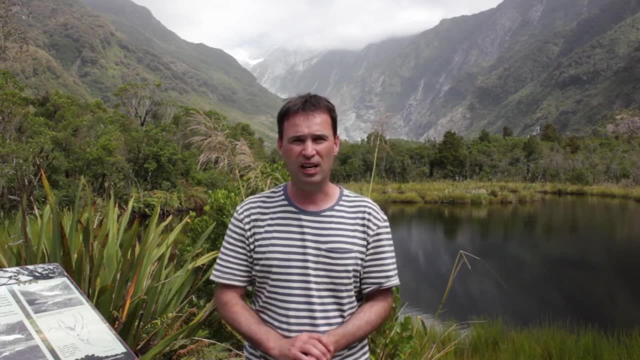 glaciations, Warmer periods, have seen glaciers in retreat and we call these interglacials. Now, at this time in history, glaciers are in retreat. Where I'm standing here at, the Franz Joseph glacier was actually once hundreds of metres under ice. 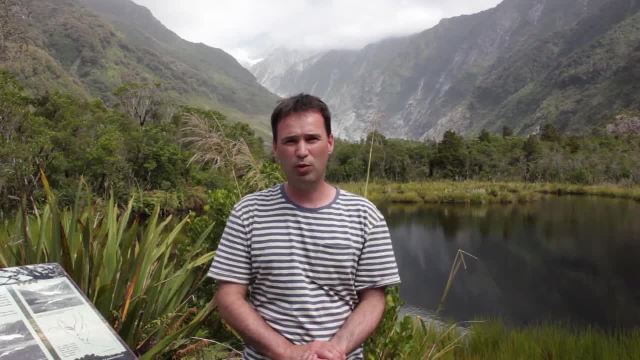 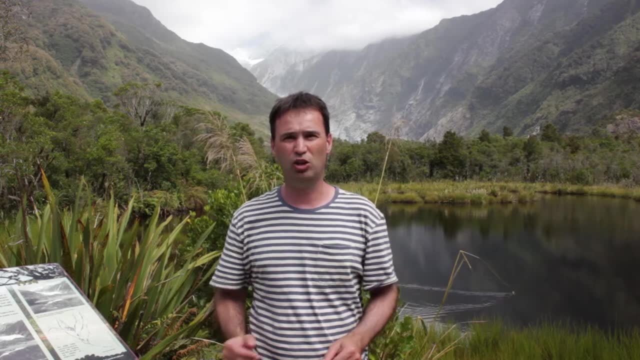 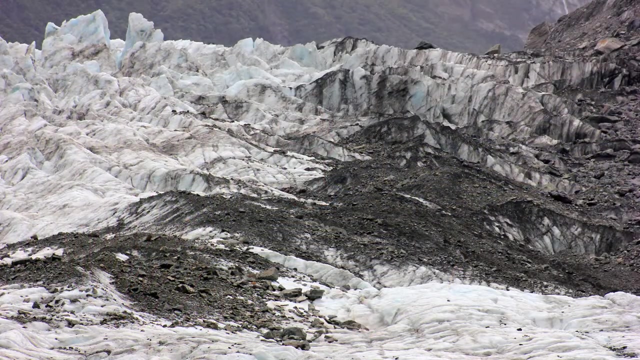 me this pool, which is known as Peter's pool. It is what we call a kettle pool, and what it is. it is formed when a glacier that is in retreat leaves behind a huge iceberg and eventually that iceberg melts and forms this pool. The tremendous weight of the ice combines with gravity to cause 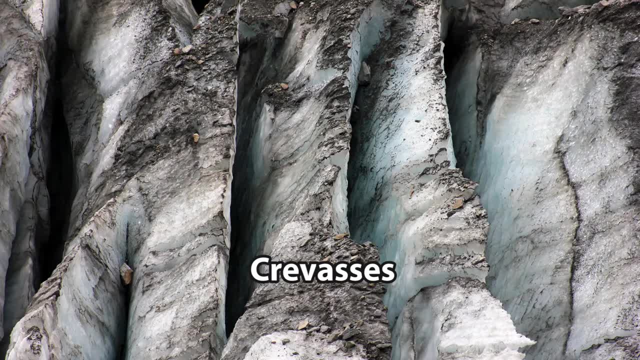 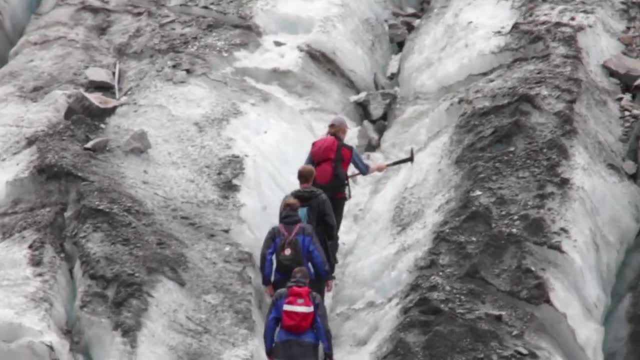 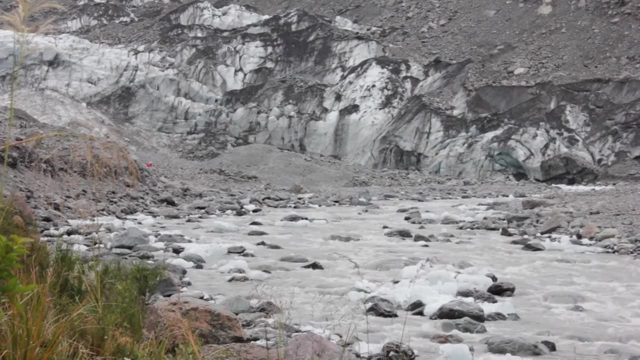 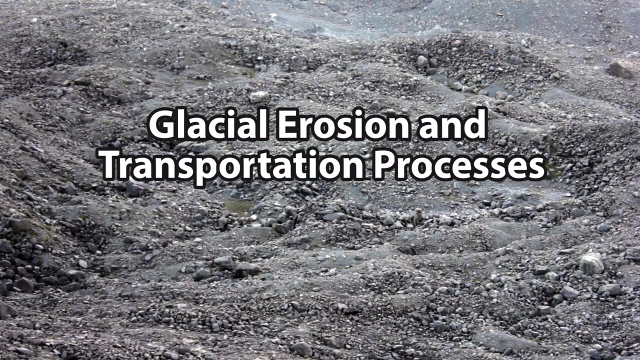 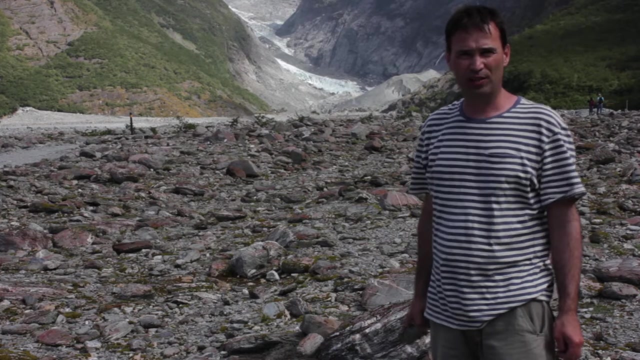 the glacier to move. At locations where glacier flows rapidly, cracks called crevasses form. Crevasses are very dangerous to climbers and should be avoided. The terminus of a glacier is also very dangerous. As glaciers move, glacial erosion processes take place, causing the glacier to transport huge 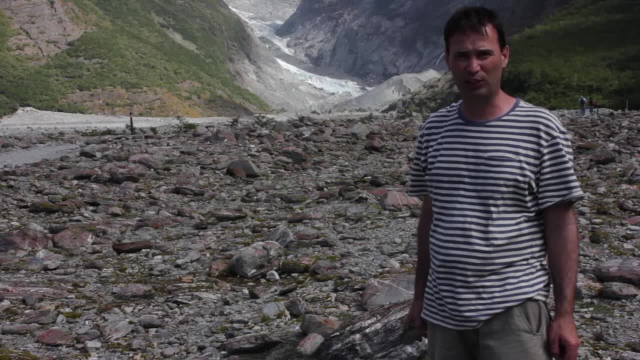 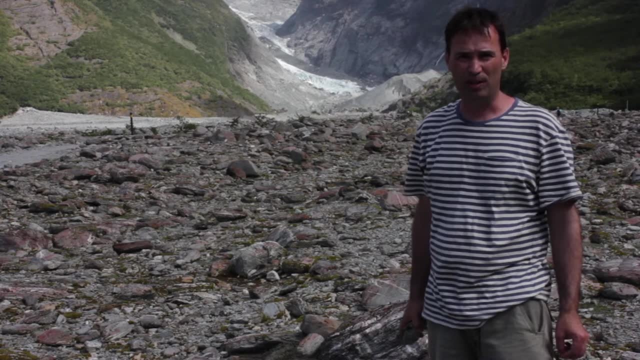 amounts of material with them. The main erosive processes of a glacier are called plucking. As the glacier moves along the valley, the ice melts slightly around the boulders before refreezing them. As the glacier moves in, the boulders are then ripped out of the ground. 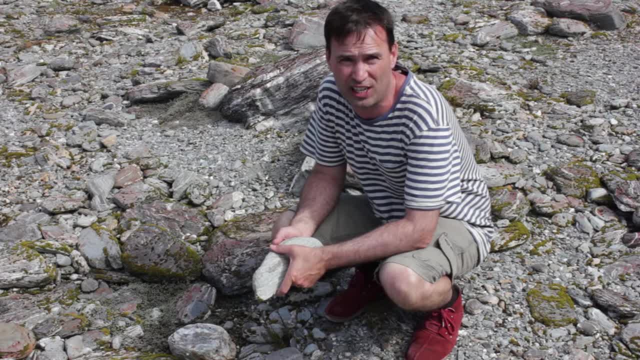 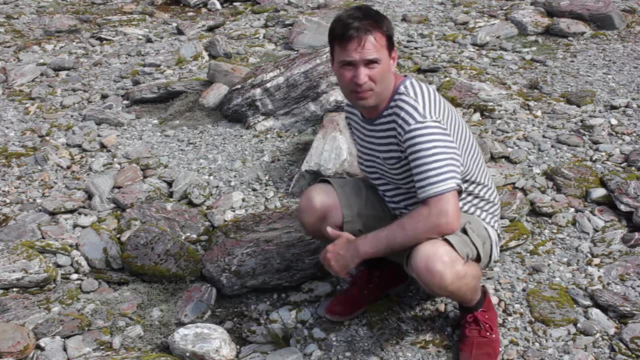 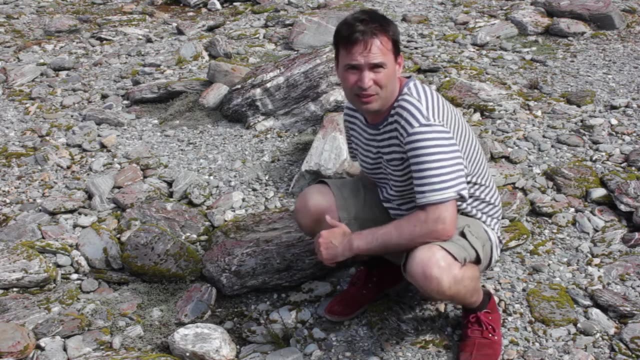 Any rocks and boulders embedded in the bottom and sides of the glacier become agents of the process of abrasion. These rocks glide against the bedrock and rock faces of the glacier as it moves, Just like a glacier sandpaper. the grinding of rocks against the bedrock causes the wearing away of the landscape. 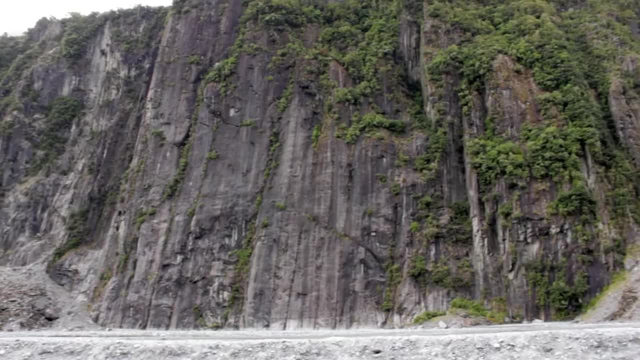 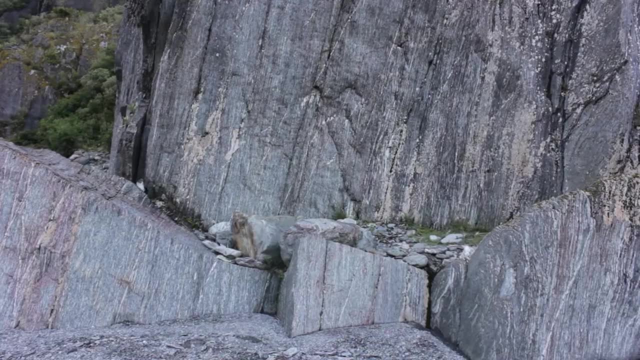 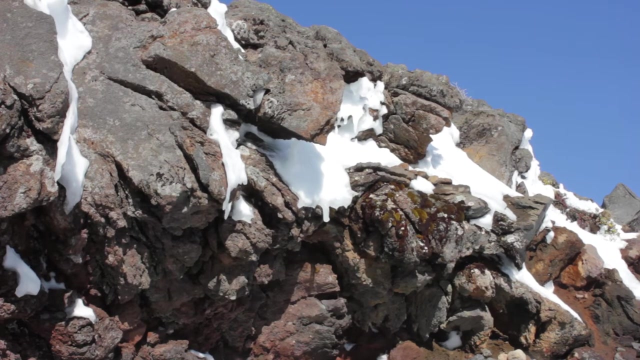 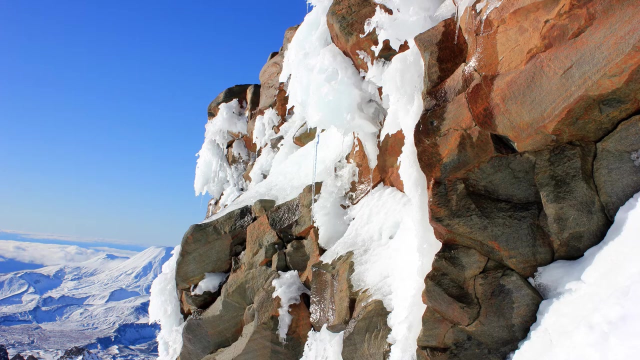 These abrasion processes leave behind smooth, polished surfaces. Sometimes these surfaces have scratches in them, called striations that have been carved out by debris embedded in the base of the glacier. Another glacial erosion process is that of freezing and thawing. Water enters cracks in rock during the day. Overnight temperatures plummet and the water freezes. 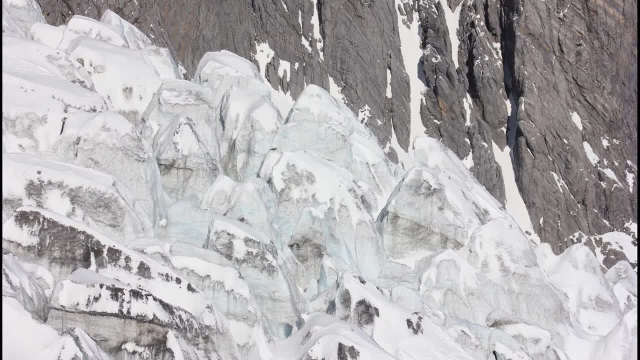 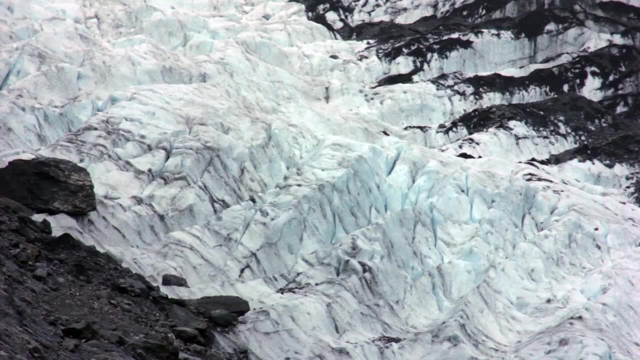 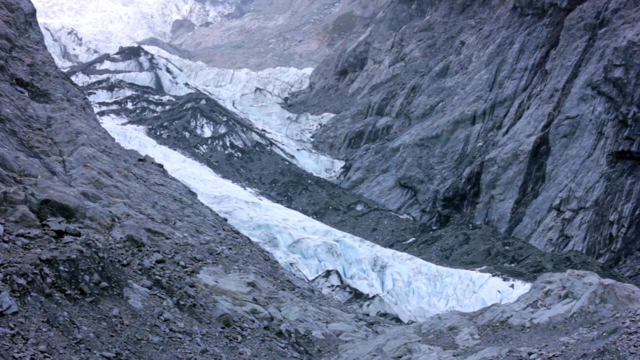 When water freezes, it expands, placing pressure on the surrounding rock. Over time, this pressure in the rock causes it to crack and split. This process makes the rocks more vulnerable to being plucked by the glacier. Glaciers transport enormous quantities of debris. Most of the material is carried near 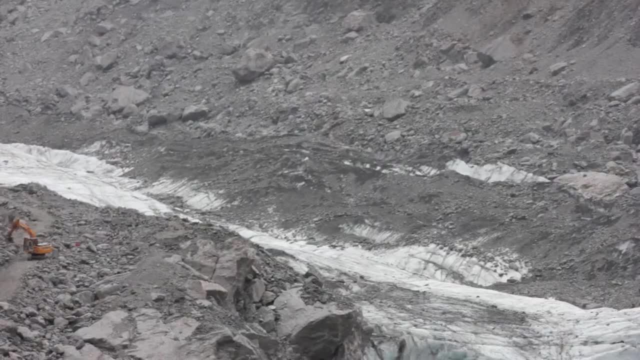 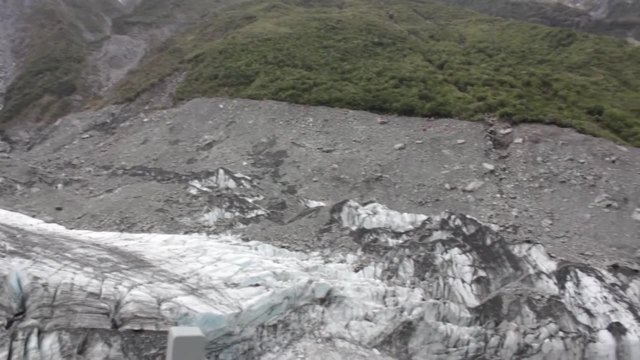 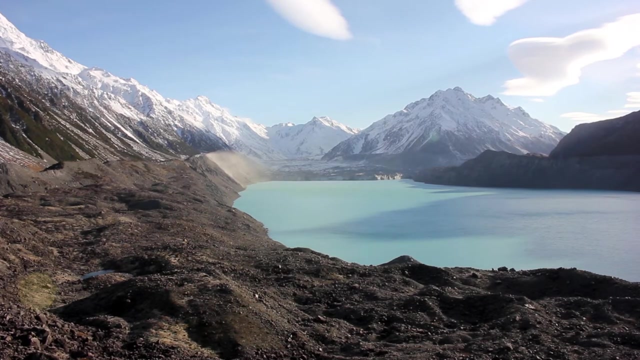 the base of the glacier From where it was plucked. But glaciers also carry frost shattered debris which has fallen from the valley walls onto the ice. It is easy to observe the debris being carried by glaciers Over time. glaciers can transport debris long distances. Sometimes glaciers split at the end. 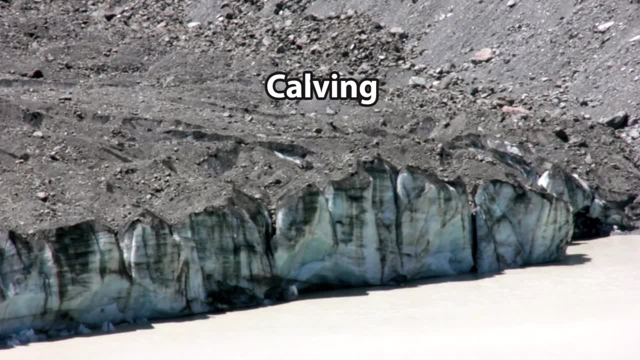 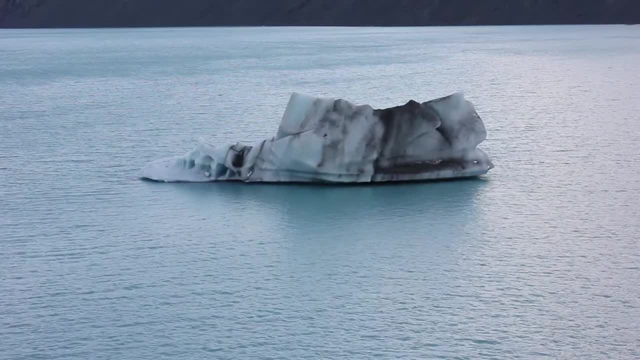 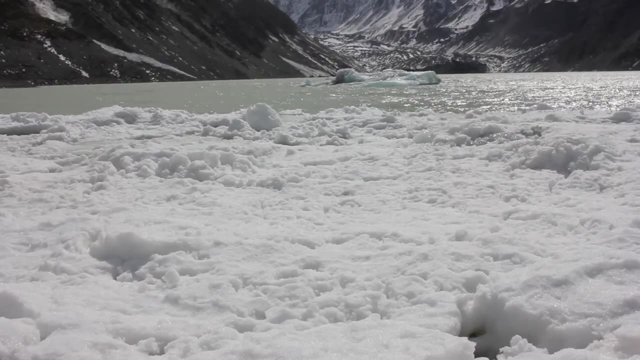 into smaller sections. This is called carving. These have potential to become icebergs if the glaciers now ends in the sea. An hour and a half walk to the Hookah Lake in the Mt Cook National Park will reward the hiker with views of the terminus of the Hookah Glacier. Carving is taking place here and numerous small 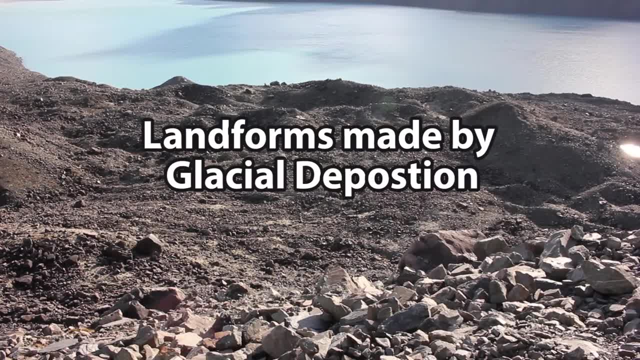 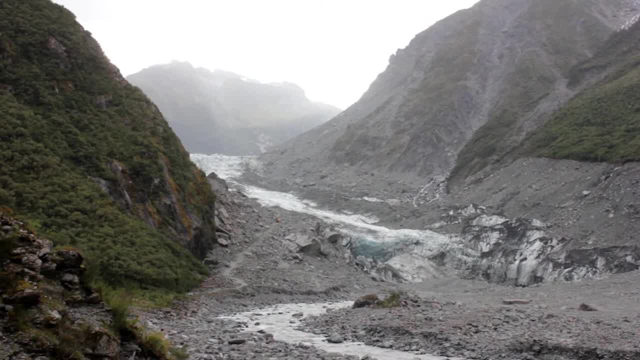 icebergs float around the lake. As glaciers reach lower altitudes, temperatures rise and ice begins to melt. As this happens, the ice cannot carry as much material as it should. The glacier is now in the middle of the lake. The main deposition features of glaciers are called moraines. 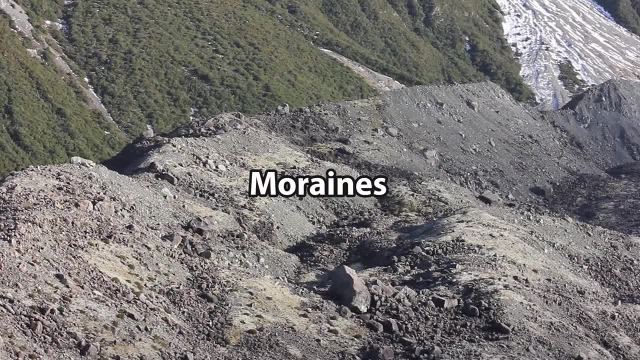 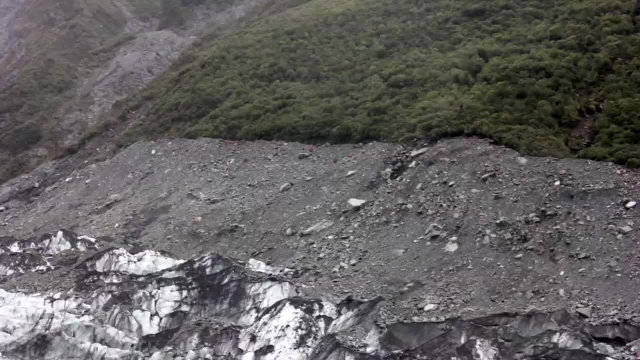 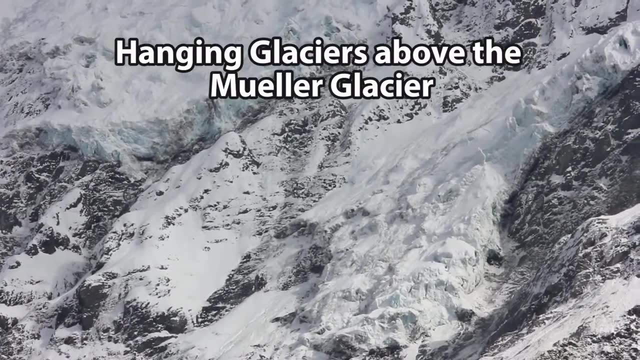 The long dark bands of debris are visible on top and along the edges of glaciers. The material on the sides of the glacier are called lateral moraines. On the walls of many glacial valleys are hanging glaciers which descend only partly to the main glacier before stopping at a cliff. 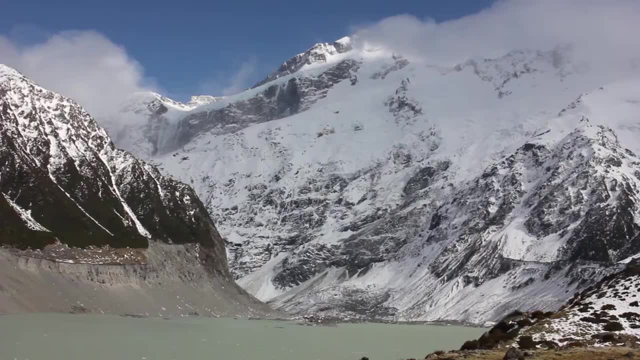 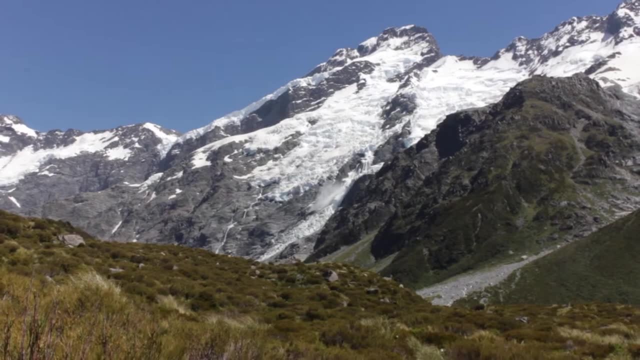 These glaciers at Mt Cook National Park are called lateral moraines. The main deposition features of the glacier is the terminal moraine. These glaciers at Mt Sefton lie above the larger Mule Glacier. Avalanches and icefalls are common here and transfer snow and other debris to the Mule Glacier. 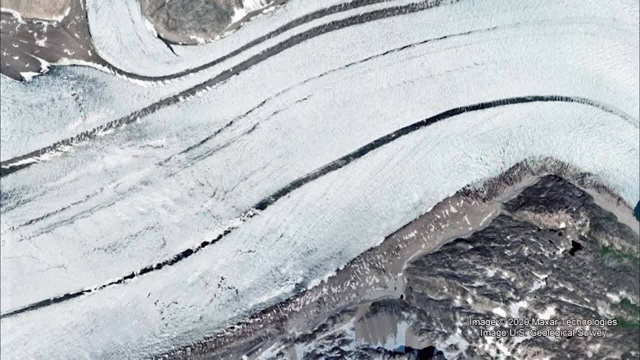 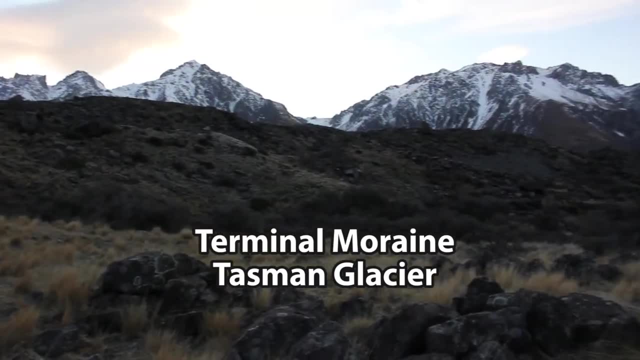 Where two glaciers emerge. their lateral moraines meet in the middle of the larger combined glacier to form a medial moraine. The main depositional feature of a glacier is the terminal moraine. This is the material deposited at the terminus of the glacier, at the 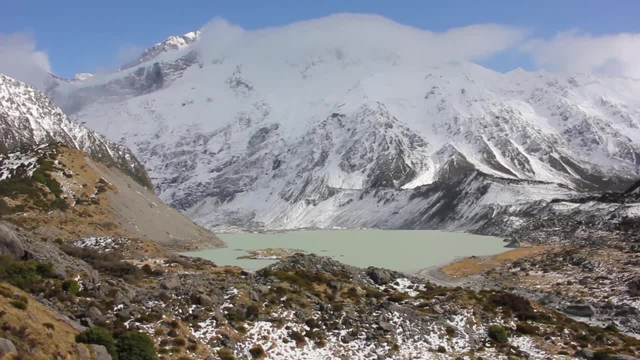 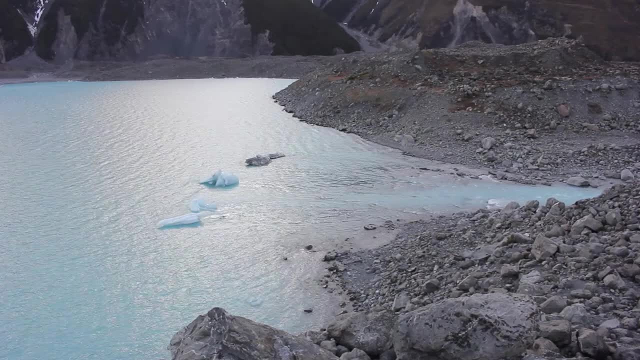 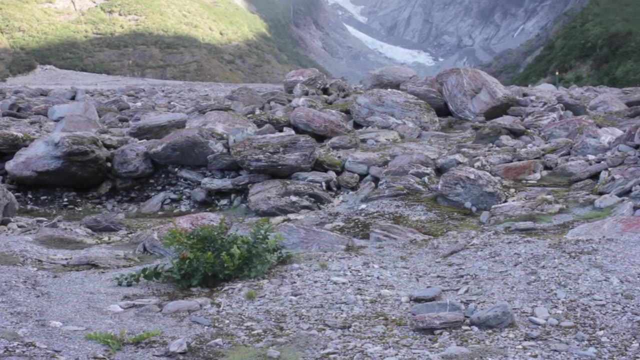 furthest extent of its growth. The terminal moraine may act as a dam for a ribbon lake At the Tasman glacier. the terminal moraine has acted as a dam, creating the Tasman lake. Glaciers deposit a mixture of unsorted clay, sand, stone and boulders. The stones are angular. 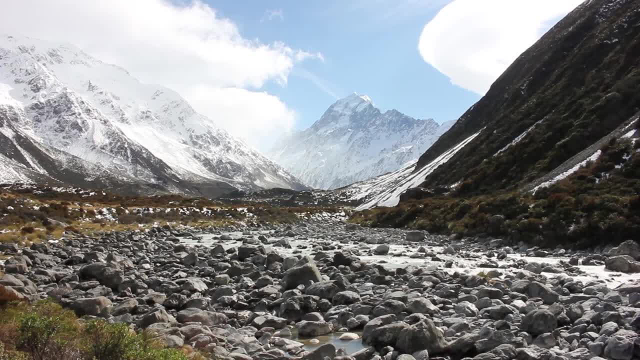 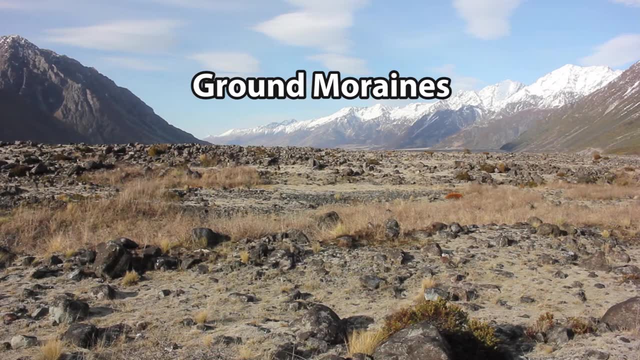 because they have not yet been rounded by fluvial processes. This material is known as till Glaciers deposit, a mixture of unsorted clay, sand, stone and boulders. 2. Glaciers depositmanares: till on valley floors to form ground moraines. Ground moraines often have a 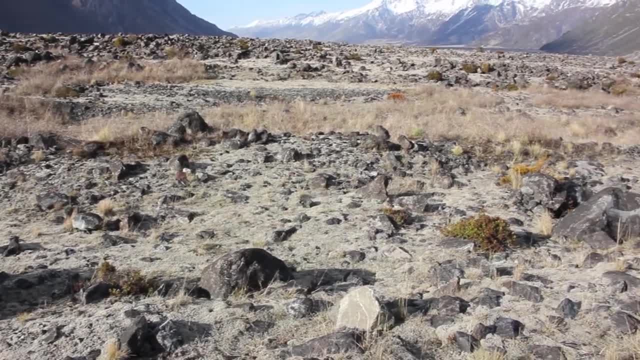 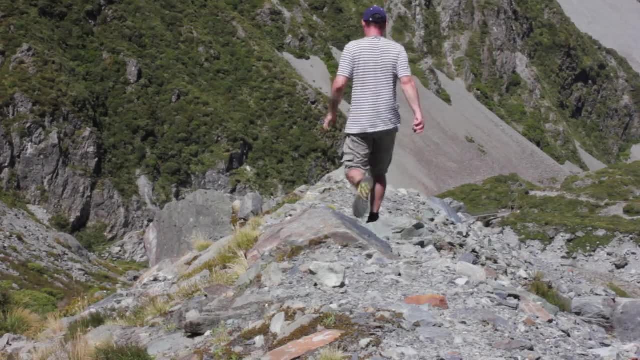 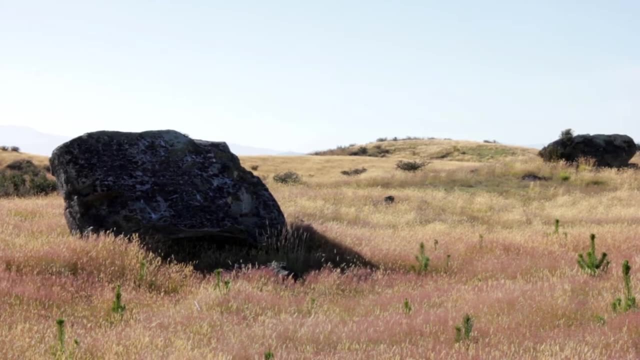 hummocky appearance and can go on to form rolling hills and plains. Climbers have to take great care when near moraines, as there is the constant danger of rock slides. Another deposition feature is an erratic. An erratic is a boulder transported and deposited by a glacier having a lithology or rock type. 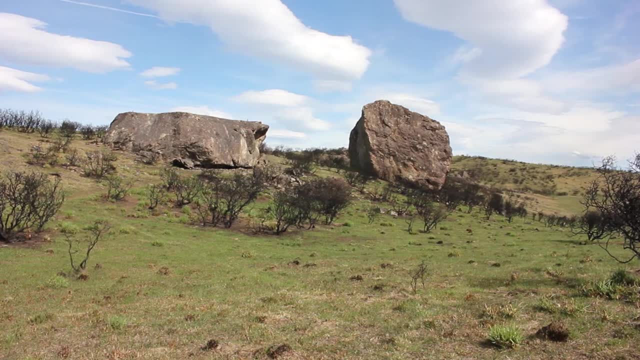 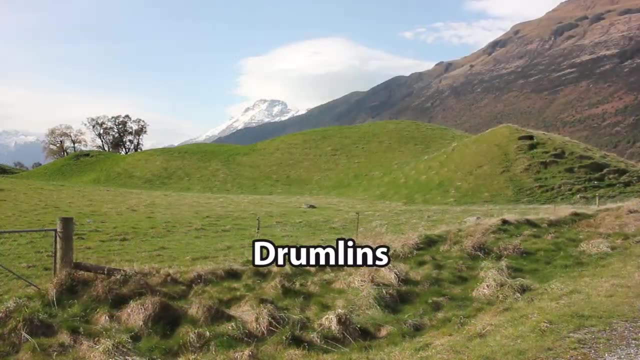 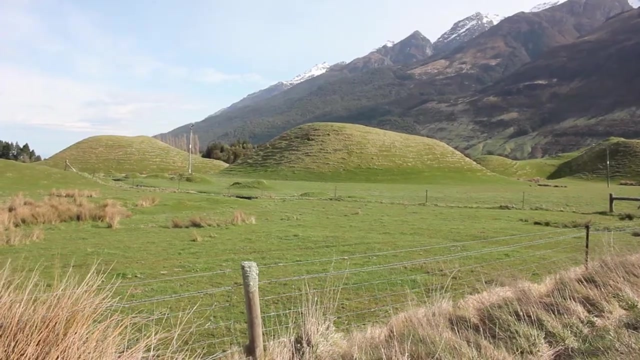 that is different from the bedrock upon which it is sitting, For example, these erratics in the Pukaki Scenic Reserve. Glaciers leave other deposition features also. For example, there are oval mounds of till called drumlins. They are 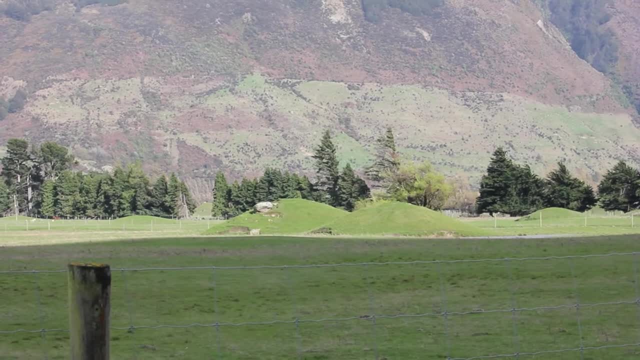 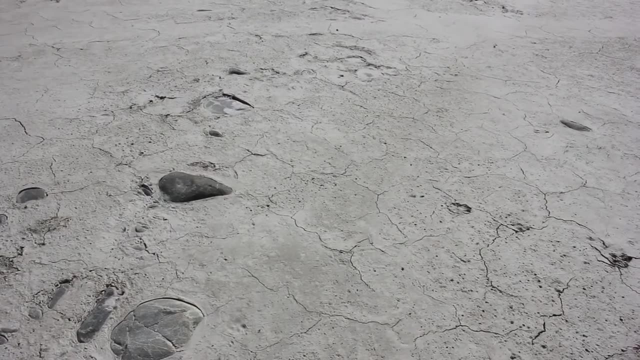 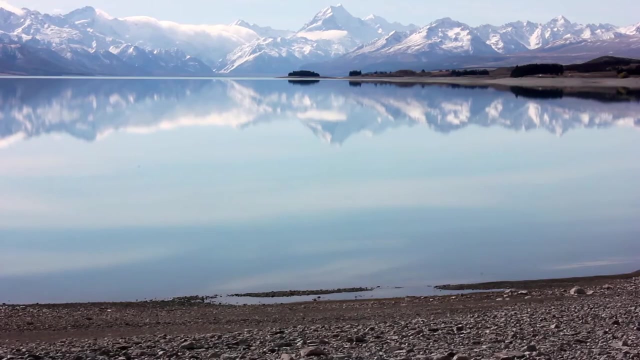 commonly found in clusters, For example, this cluster of drumlins in the Otago region. Another feature is rockflower. This is a very fine sediment. Many glacial lakes, such as Lake Pukaki near Mount Cook, have a milky turquoise color due to glacial rivers. 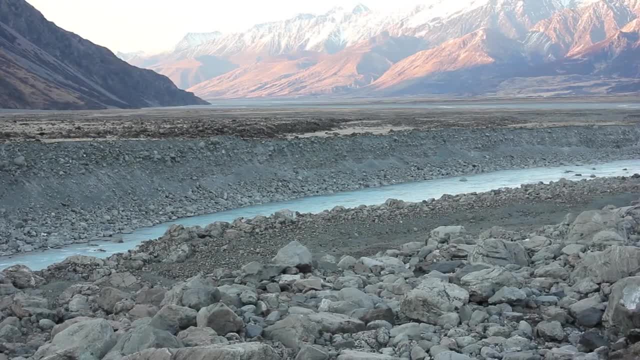 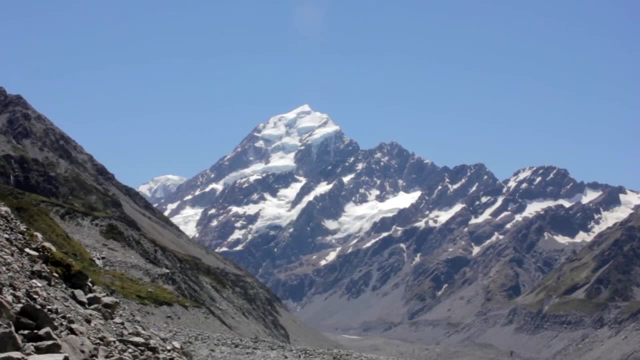 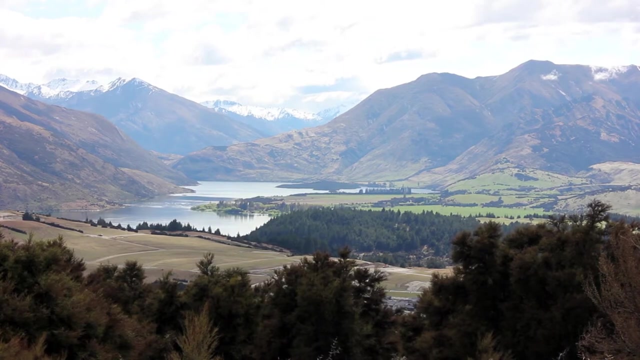 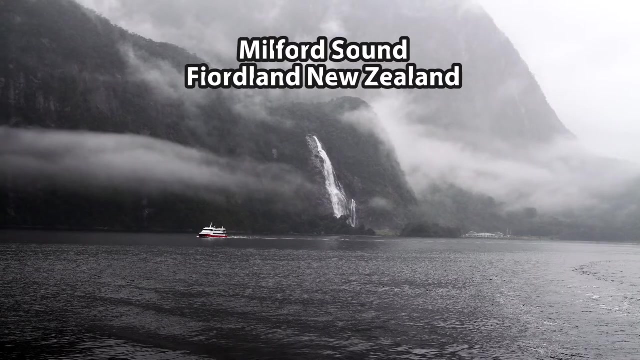 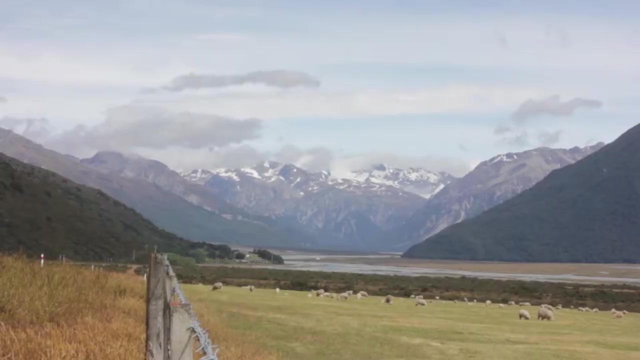 washing the sediment into them. Glacial erosion carves out a variety of landforms. Even in regions where there are no glaciers, many landforms are still found. The South Island of New Zealand has hundreds of fjords, ribbon lakes and U shaped valleys that exist as reminders of the giant glaciers that once were there. 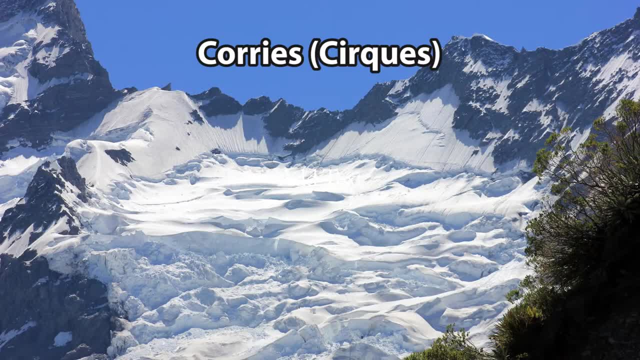 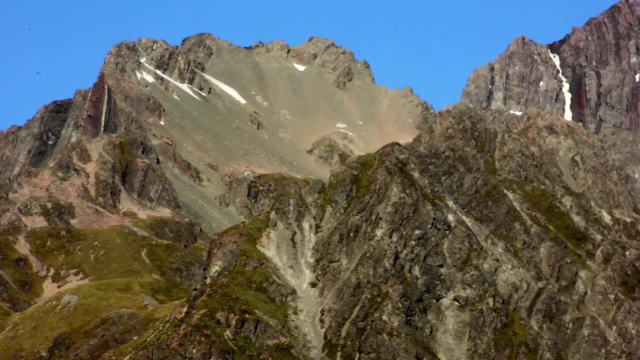 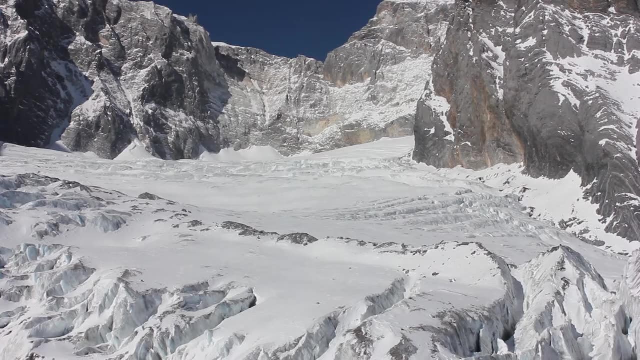 A Kohie, also known as a cerk and nitikan, is an erosion feature formed at the starting point of a glacier. Kohies have a rounded hollow with a steep backwall. Corries form when snow accumulates in hollows on mountainsides, slowly accumulating enough to turn into ice. 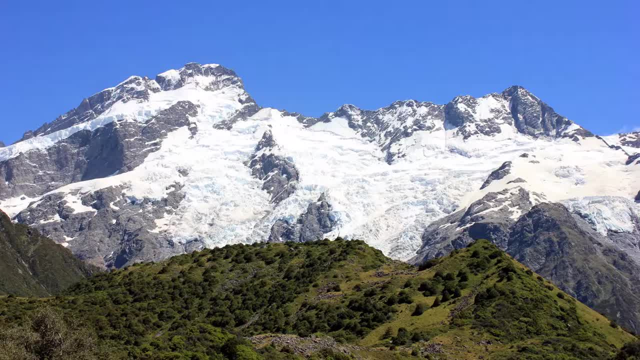 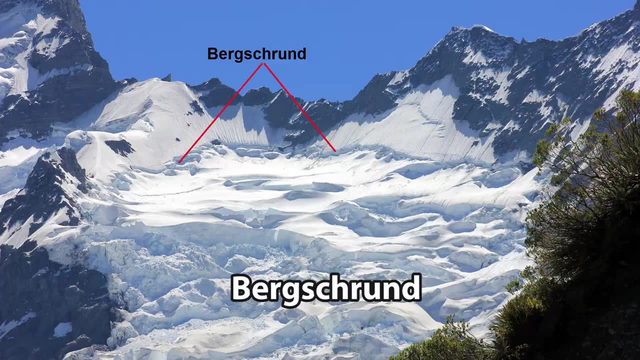 This ice slowly gouges out a steep back wall through the processes of freeze thaw and plucking. Large crevasses on the top of the ice, called a birch crumb, allows water to flow onto the ice, where it freezes to create more ice. 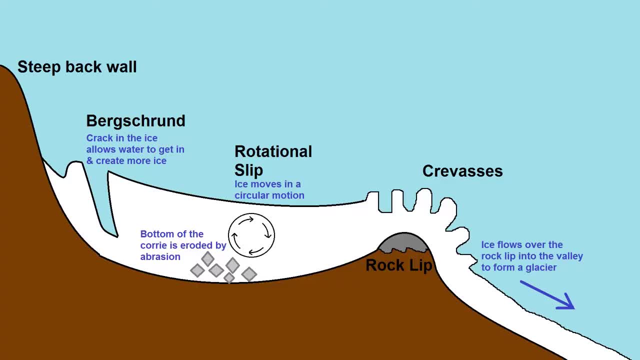 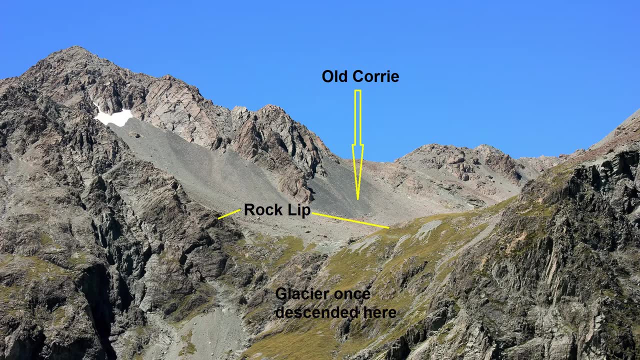 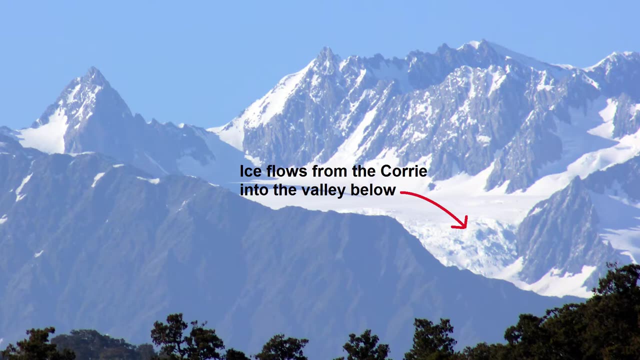 The bottom of the curry is eroded by abrasion as the ice moves in a circular motion known as rotational slip. At the front of the ice, the erosion is less causing a lip of rock to be left there. As more ice accumulates, it flows over the lip and into the valley below, forming a glacier. 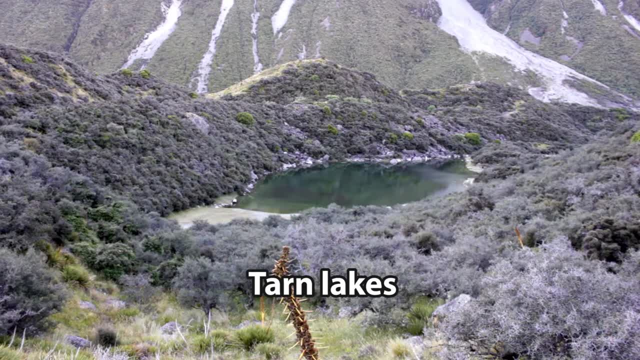 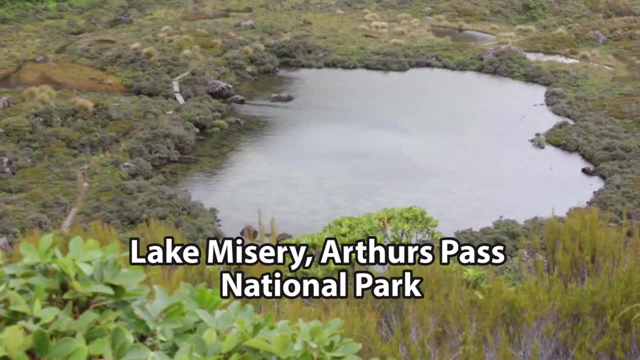 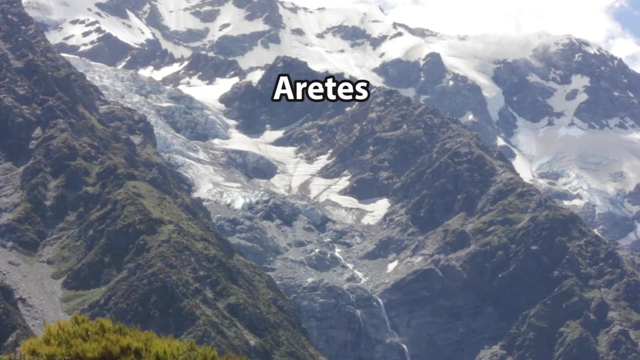 In places where glaciers have retreated, the curry was often filled by meltwater to form a lake. The rock lip in the bottom of the ice moves in a circular motion, known as rotational slip. These lakes are known as tarns. When two curries form back to back, they both erode backwards until they create a narrow, knife-edge ridge between them. 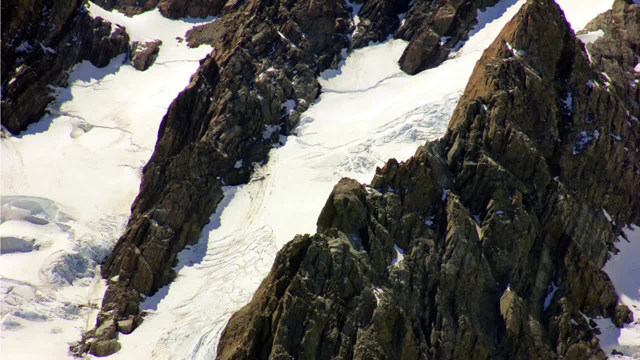 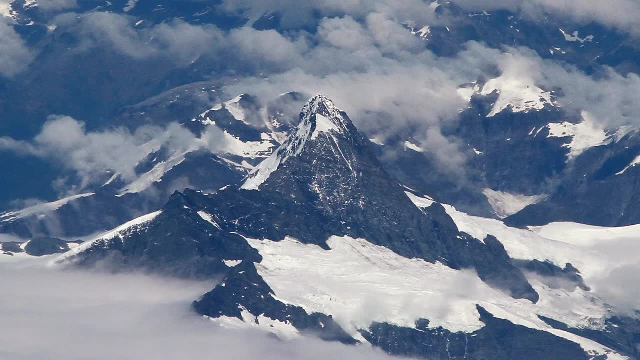 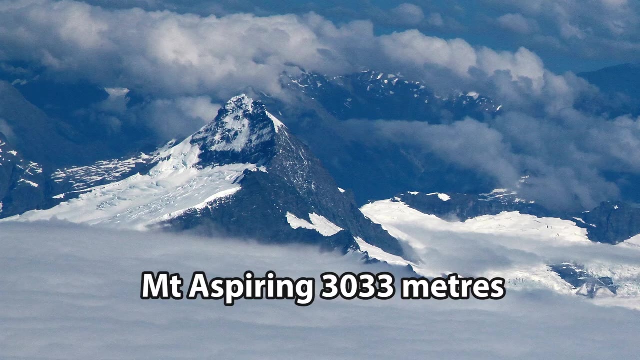 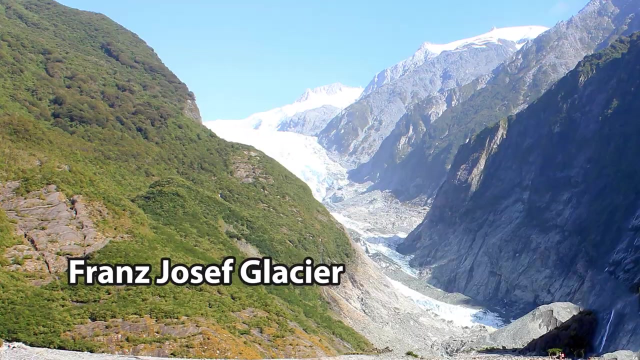 These sharp ridges are called aneretes, Sometimes three curries back into each other. They eventually erode backwards to leave a sharp pyramid peak. An example of this is Mount Aspiring in the Southern Alps of New Zealand. Glaciers carve out U-shaped valleys, just as a river produces a V-shaped valley. 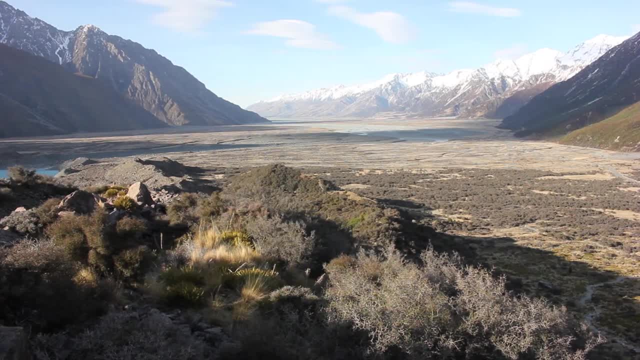 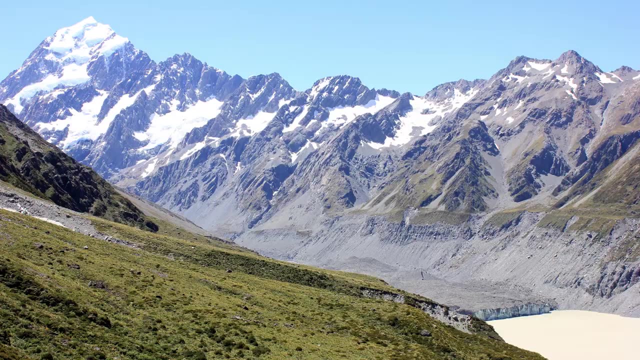 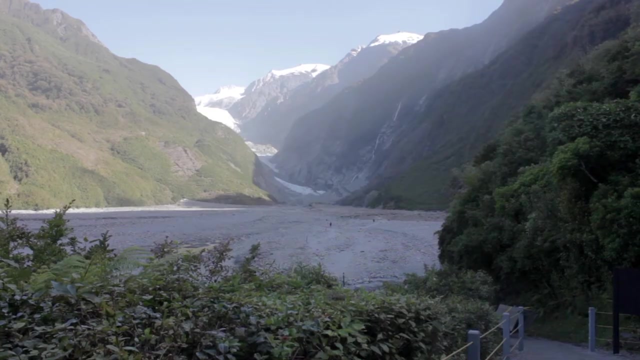 Usually, a glacier will follow the general direction of a river valley, but instead of flowing around areas of hard rock like a river does, a glacier will cut straight through it. This means that when the glacier melts, it leaves behind a U-shaped valley with very steep sides. 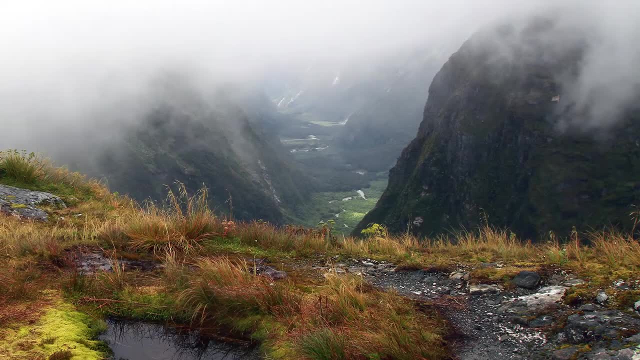 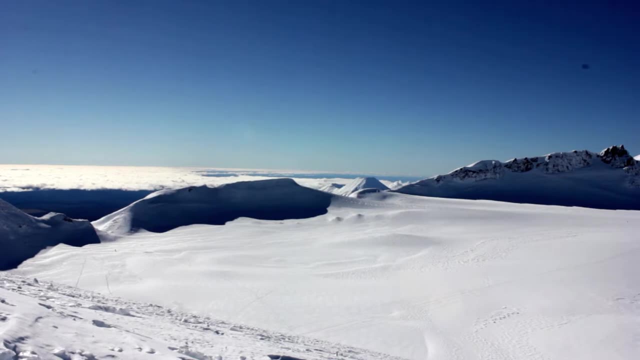 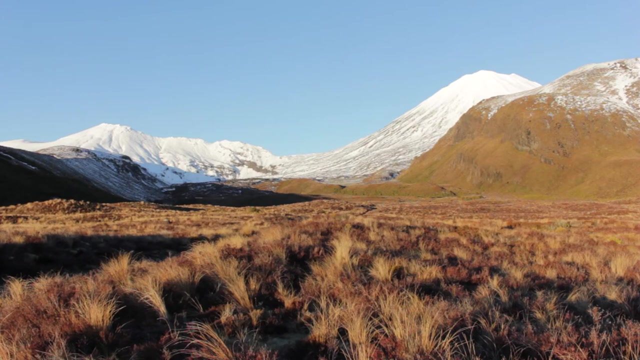 There are numerous U-shaped valleys in the South Island of New Zealand. The warmer North Island only has small glaciers, on the summit of Mount Ruapehu, for example, the Whakapapa Glacier seen here. However, at Mt Tongariro you can see the evidence that larger glaciers once existed here. 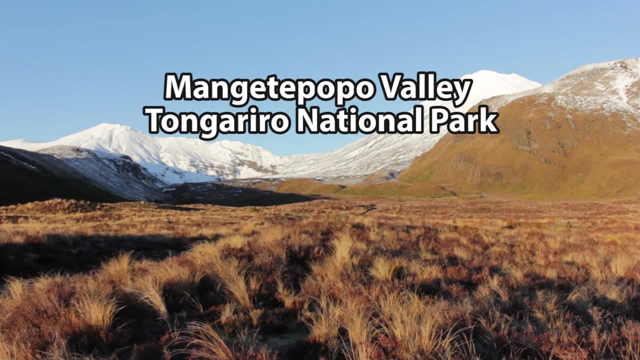 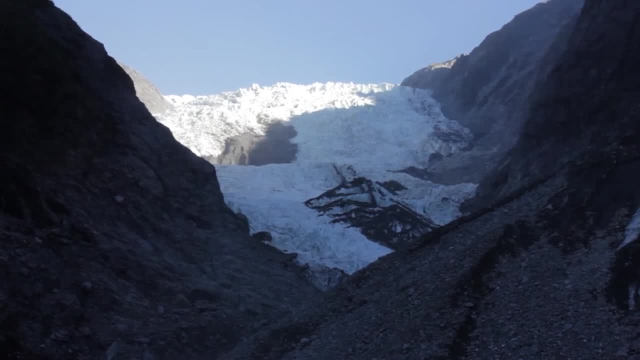 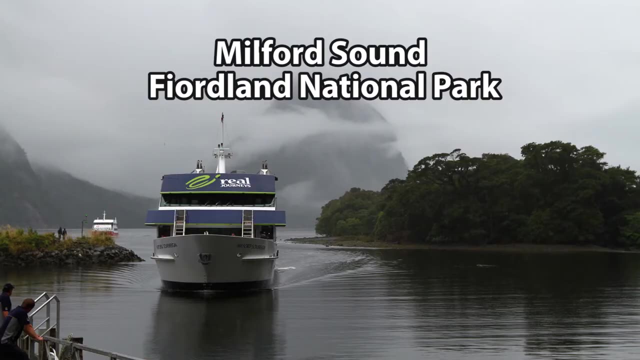 in the form of the U-shaped Mangatapopo Valley. Some glaciers, such as the Fox and Franz Joseph Glacier, descend to low altitudes not far from the Tasman Sea. When global temperatures and accompanying sea levels rise, low-lying U-shaped valleys get filled with water to become a fjord. 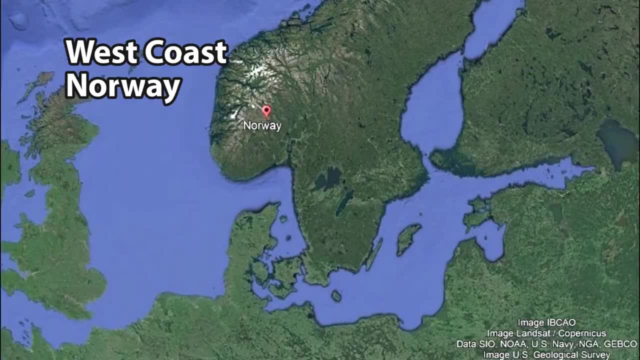 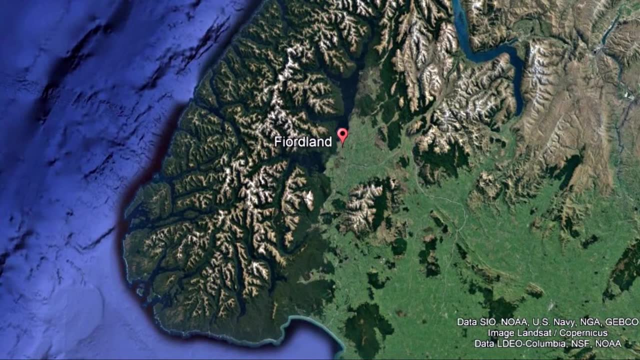 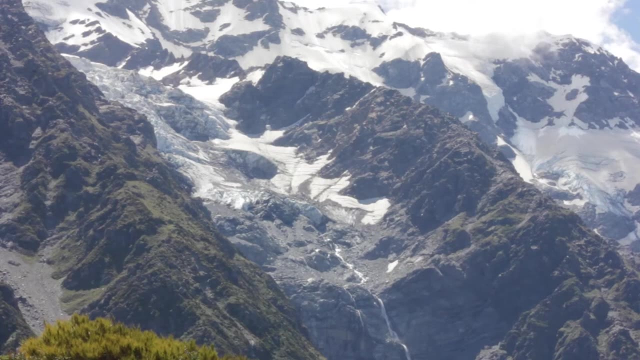 This produces a coastline with an irregular shape, like those also found in Norway, Western Canada and Fjordland, New Zealand. Another feature associated with valley glaciers are hanging valleys. The floors of the tributary valleys are eroded at a slower rate than the floor of the main valley. 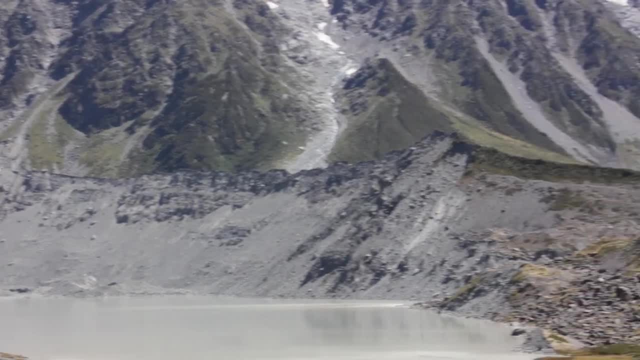 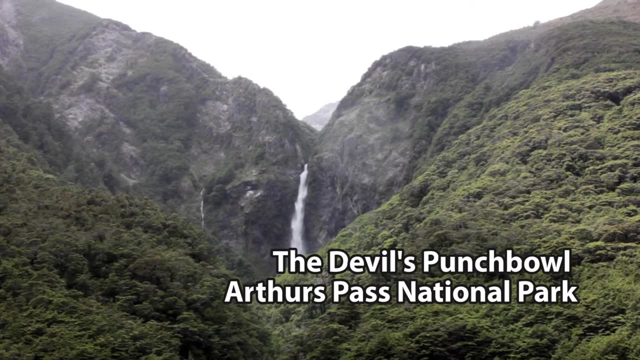 so the difference between the depths of two valleys steadily increases over time. The tributaries are left hanging high above the main valley, with their rivers and streams entering the main valley by means of either a large waterfall or a series of smaller waterfalls. 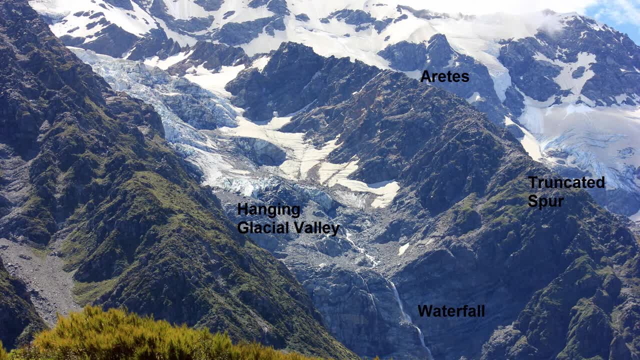 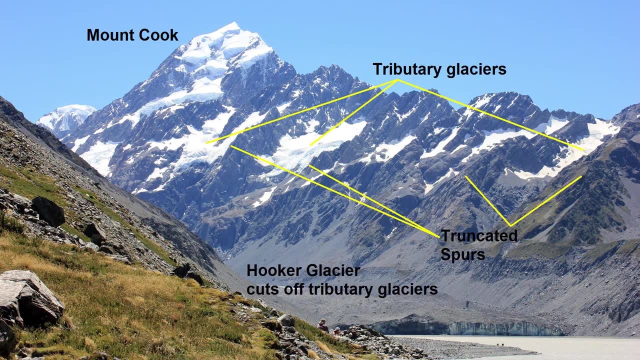 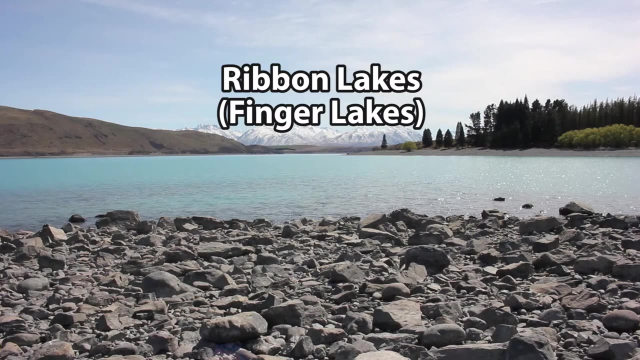 The valley sides may also have truncated spurs, which are the ends of sloping ridges that have been cut off or truncated by the valley glacier, which flows straighter than a river would. You can see these features in this diagram. Finally, retreating glaciers leave behind ribbon lakes on the valley floor. 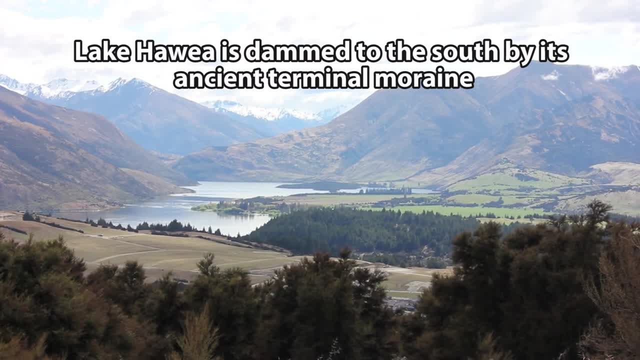 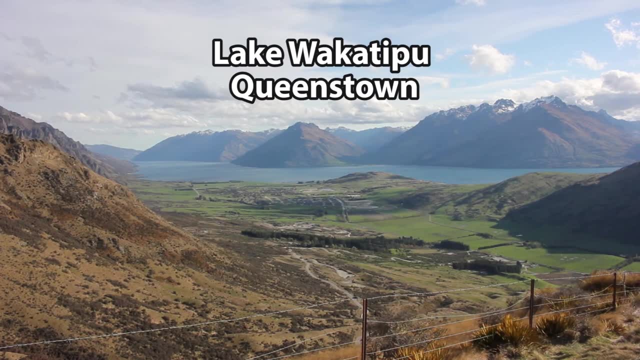 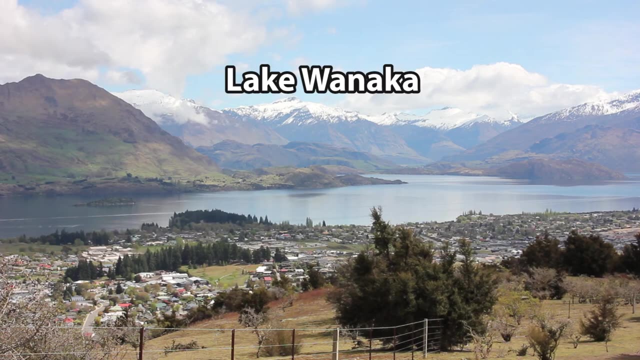 with the terminal moraine acting to form a dam to hold the water in. These are also known as finger lakes because they are long and narrow. The South Island has numerous lakes that fill deep valleys, excavating the glaciers, For example, the 42km Lake Wanaka. 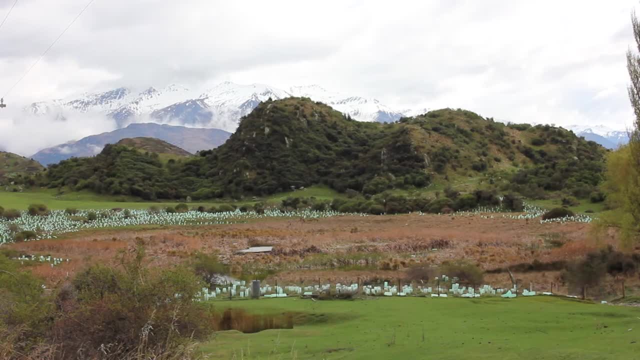 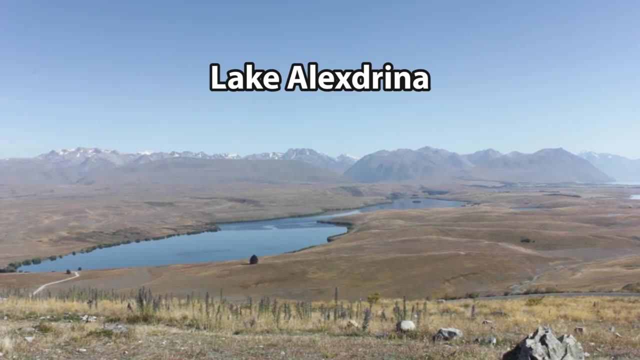 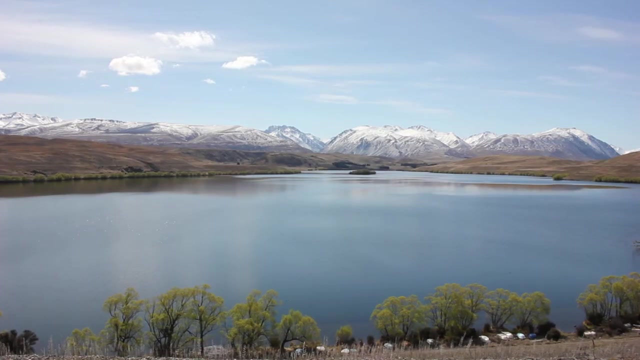 which lies in an ancient U-shaped valley. The ancient terminal moraine encircles the lower end of the lake. A smaller example of a ribbon lake is Lake Alextrena in the Mackenzie Basin. This lake has been enclosed behind moraines left behind by an ancient glacial advance. 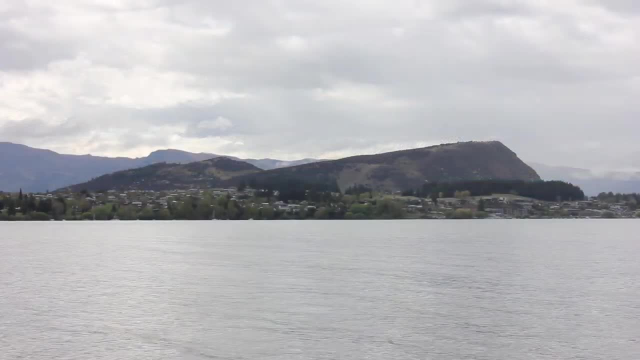 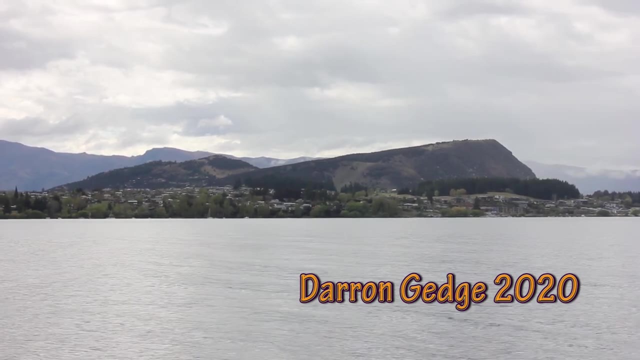 Lake Alextrena is one of the most beautiful lakes in the world. It is the second largest lake in the world. Lake Alextrena is one of the most beautiful lakes in the world. Lake Alextrena is the second largest lake in the world.